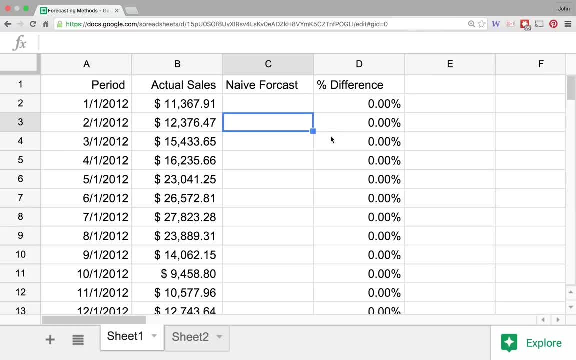 data, we'll say, okay, the naive approach of forecasting. again, if we go back to our original forecasting methods, video overview is where we take simply the previous period and we forecast and say, okay, next period we're going to do the exact same. And so what that equation would? 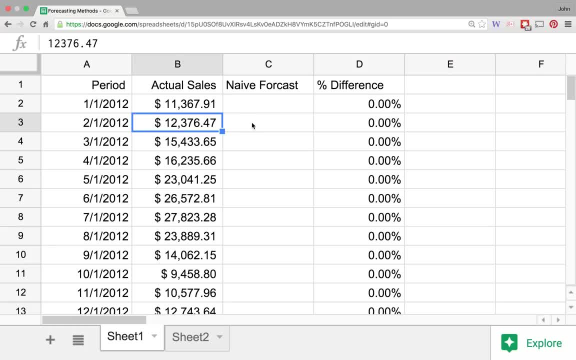 look like here is that we would take this period and we would say: okay, our forecast is going to equal the previous period. Now, over here in column D, what I've got is: I've got a percent difference And you can see the function here that I've got, And basically what it says is: 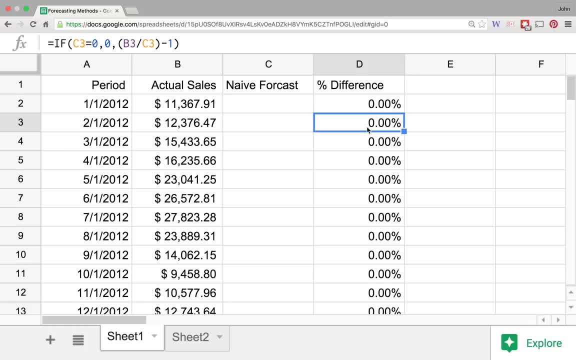 that if the forecast is less than the actual sales that we see in that time period, then that number is going to be a positive number. So it's going to say, okay, our actuals were actually greater than what we forecasted. And if it's the other way around, of course we'll see a negative. 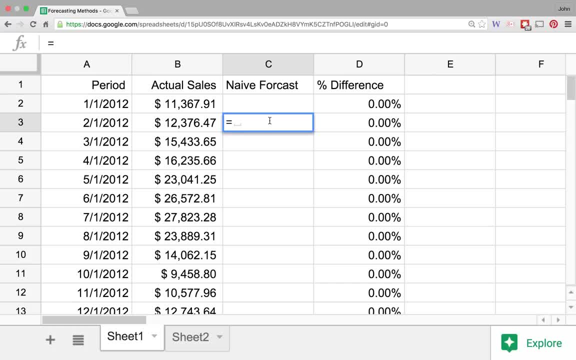 And so let's take a look at the naive method of forecasting. So let's take a look at the naive approach of forecasting. We take the current period and we'd say, this period, our forecast is going to be equal to the last period, And then we'll go through and we'll drag this down. 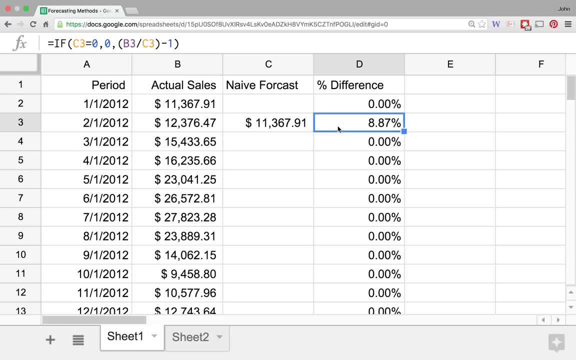 here in just a minute. So our very first period that we look at, we say, okay, well, we're within a 10% difference and it was kind of in the right direction, right. So sales were going in a good direction. They were a little bit better than we had. That might present maybe some inventory. 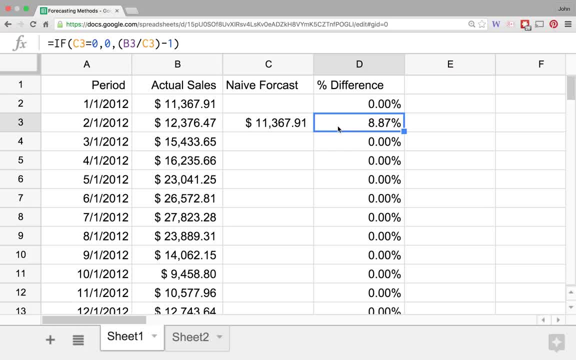 issues with us under forecasting what we think is going to be super important. So we're going to say, well, we're going to be sold in this upcoming period. So let's take a look at how the naive forecast would work if we were to use the naive forecast through all the periods for this three. 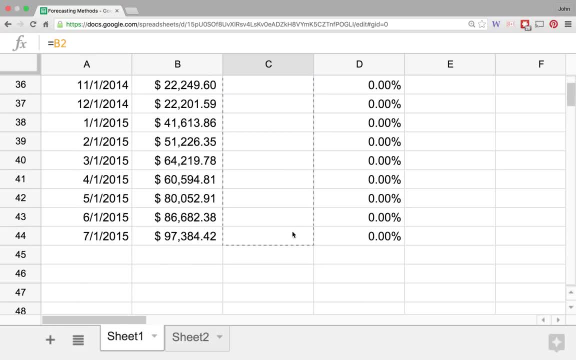 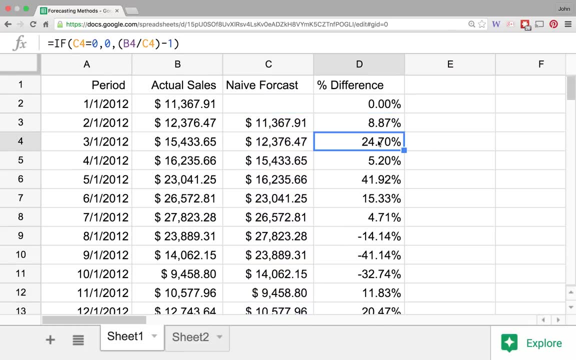 and a half year time period that we've got, And so we'll go ahead and we'll just drag this down through the three and a half year time period And we'll take a look at a couple of these things. So we start looking at it and we say, okay, wow, we're always over-performing. 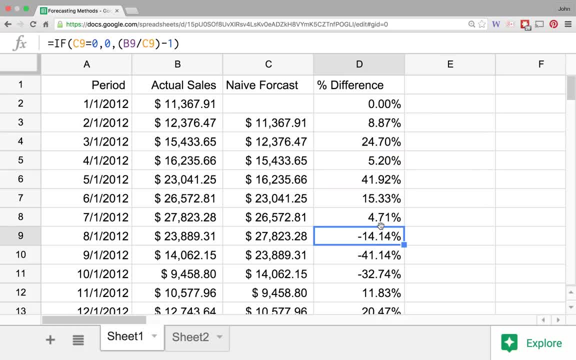 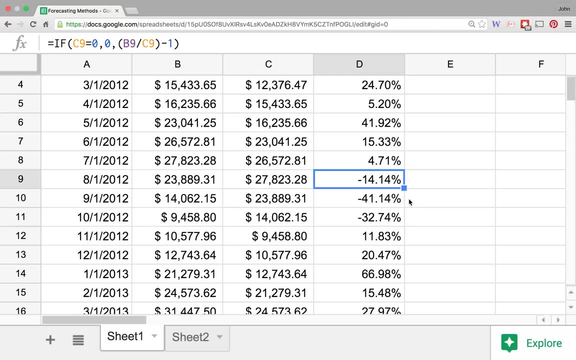 until we get, maybe, over here to period number eight, And then we start to underperform. And so we look at it and maybe one of the first things that we notice is we say, okay, we've got this positive performance. that's more than what we expected from the previous period. 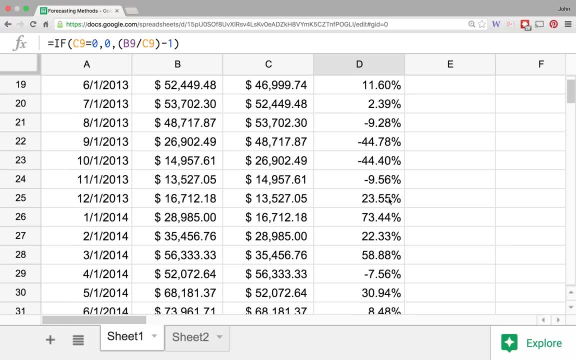 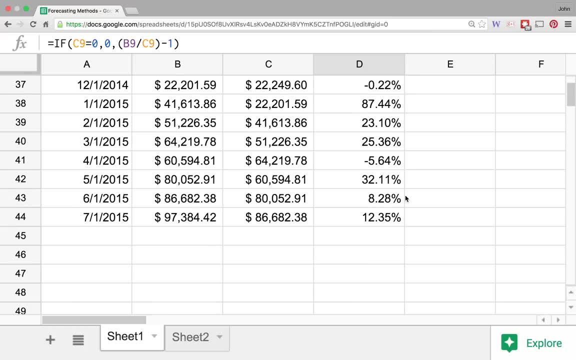 And then we've got a negative performance, Then we go back into a positive performance, And then we've got three periods of a negative or four periods of negative performance, And we continue to see that same cycle. So one of the things that might happen is we might look at that and say: 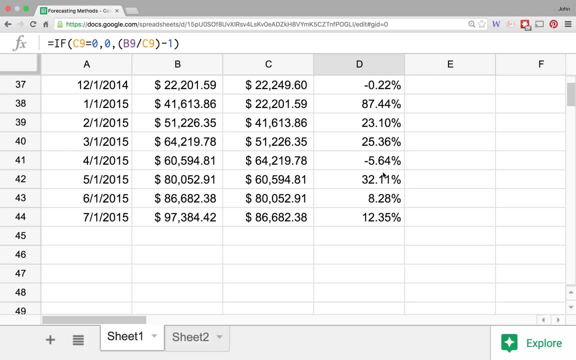 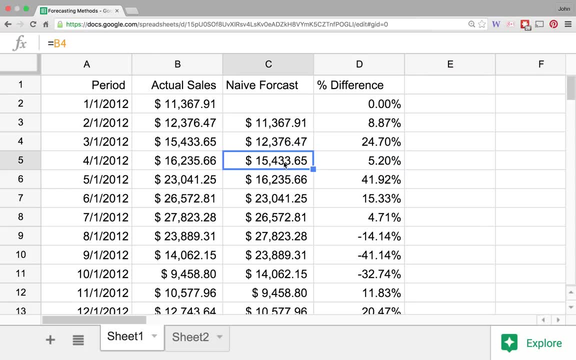 wow, this is actually a pretty strong seasonal trend that we've got here And a couple of these periods, I mean they're pretty close. We've got a 5% difference between what our naive forecast said and what we actually did. 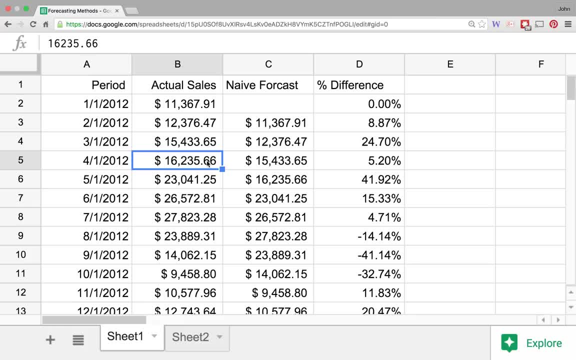 And in this one you may have a sales manager that says, hey, that's great, We underestimated what we're going to sell, And so we always like to do that. We always like to under-promise and over-deliver. But the problem is when we get into, maybe, some of these inventory issues. 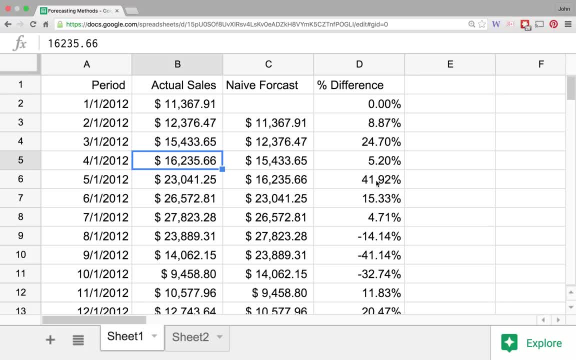 anytime that we start to see big difference or a negative difference, then we start to find ourselves in a rough situation If we're really, really under forecasting. maybe we were only able to sell 41% more because that's all the inventory that we had available on the shelves. Maybe we could have sold a lot more as a company. 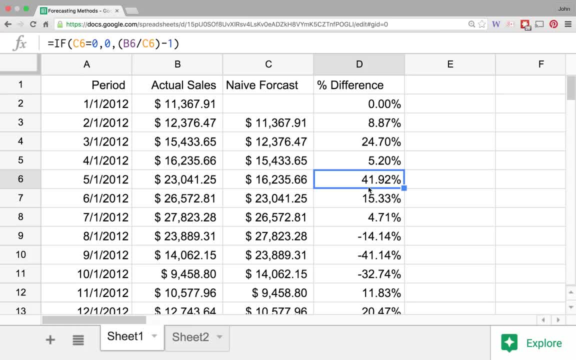 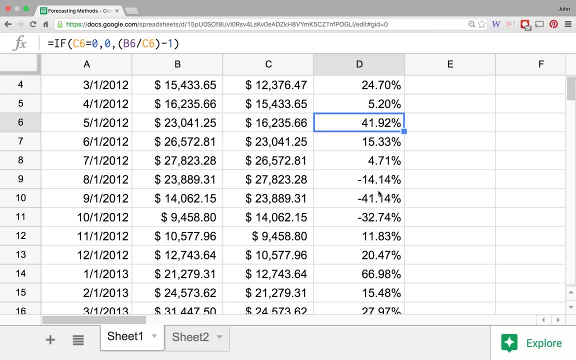 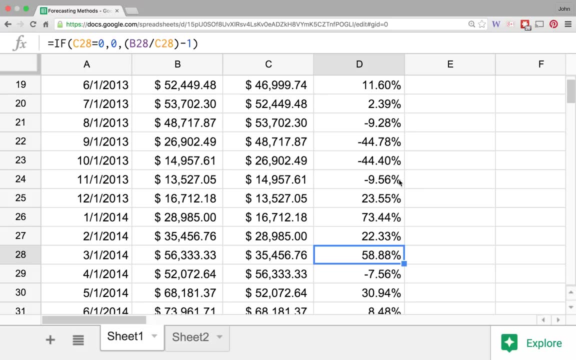 if we would have been able to accurately forecast what was happening. And so, if we look at this naive approach, we can see that there were big, big fluctuations. We had, you know, 41%, negative 41%. We come down and we see a 66%, 73%, 58%, You know. 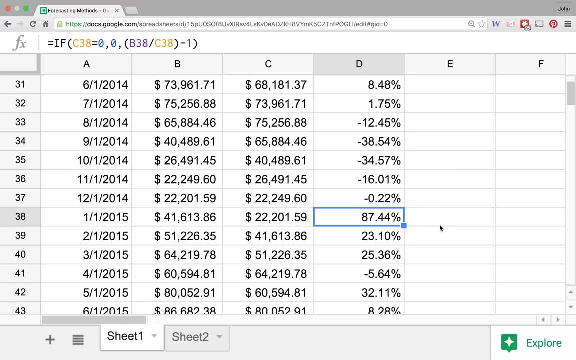 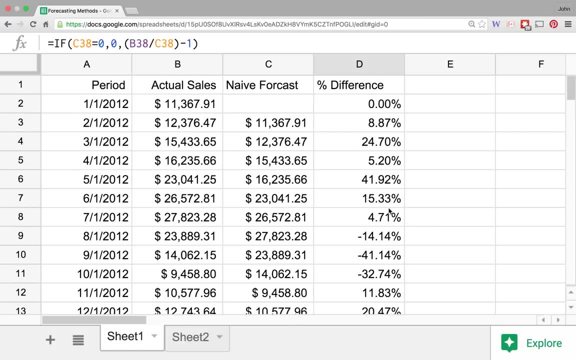 In this other case, you know the 70% was 50%. We have a lot of the same thinkings And so if you look at this method, that we looked at the 70% to 80% of the sales hit and then 81% of the sales hit, which is a real, real good percentage, we've got around 97% difference. We already have an 80%- 87% difference here as well, And then I mean clear up here: we've got an 80%- 87% difference on one of these periods. So this forecasting method. 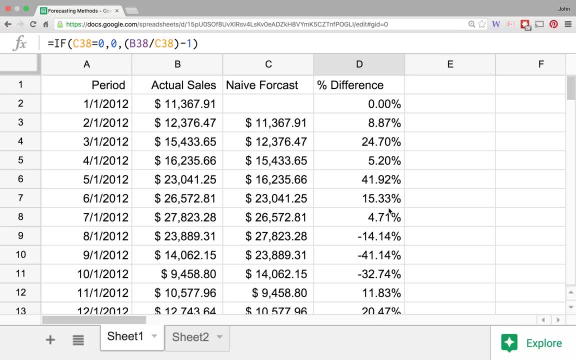 they can do next month. a lot of them forecast simply what they did in the previous month. I think I can hit that exact same number, and so we tend to see those types of forecasts that that come over from those salespeople. so again, thanks for tuning in in. in our other videos we'll talk about the other. 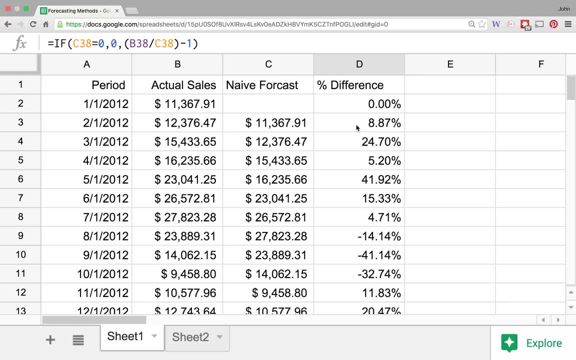 methods of forecasting. but yeah, if you have any questions or comments, leave them in the comment section below. thank you.